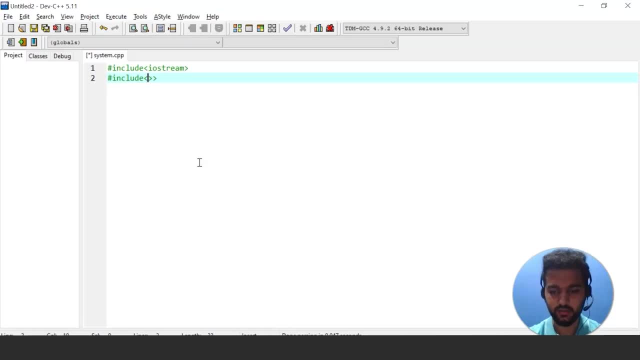 We'll add another header file which is hash, include fstream. Now the third header file which we will be adding, that would be sstream. So this fstream library, the fstream library, is used because we have to work on files and this library allows us to do so. 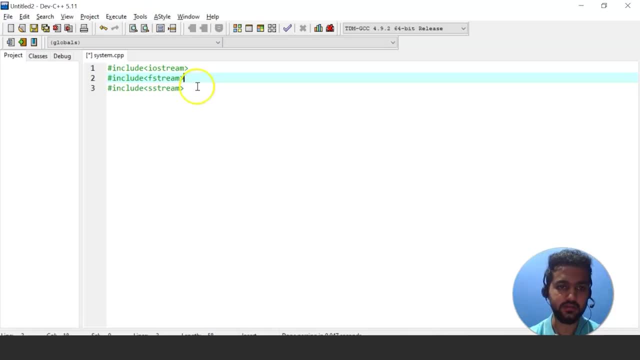 It is used for file handling operations. Now the second one, that is, the sstream library. This header file provides templates and types that enable inter-operation between stream buffers and string objects. So this was it. Now we will have to add another header file. 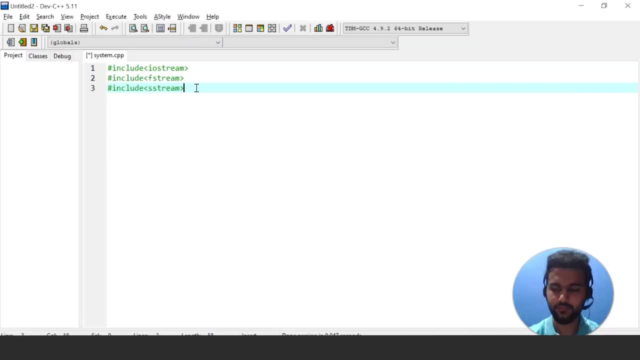 All right, Then let's do that. Hash include string. all right, So iostream, fstream, sstream and string. We have added the header files, So using namespace std- all right. Now we will create the main function, that is, int main. 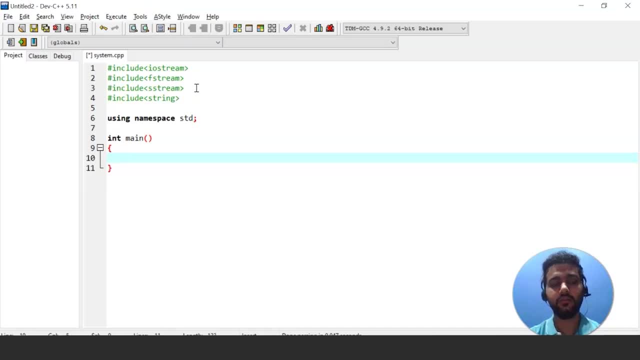 Now, inside the int main, first of all we will be creating variables. So let's do that. Int a, let's say now we'll initialize i with zero. Now we will be creating some strings, let's say string text, All these variables. 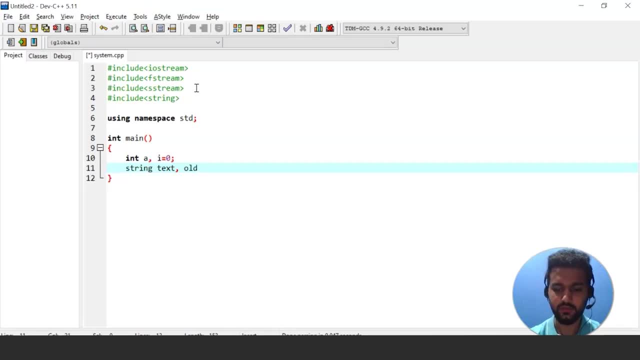 We will be using it later in the project. So let's create them Password. Let's say password one, password two. let's name it: pass name, password, zero, age, user, word age And word one. So we will be using these variables later in our project. 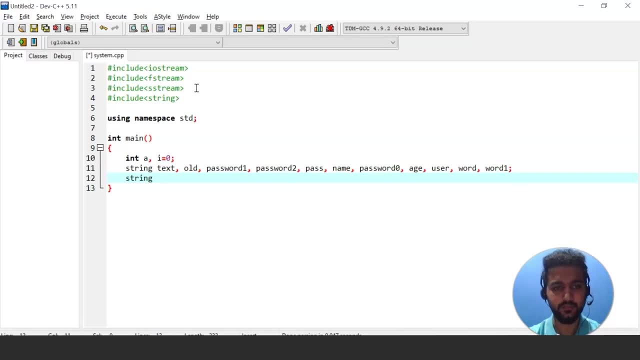 All right, Now let's create some string array. So creds, that is credentials. we'll make an array right. cp two. all right, Now we'll decide what we're going to use. We're going to use cp two. 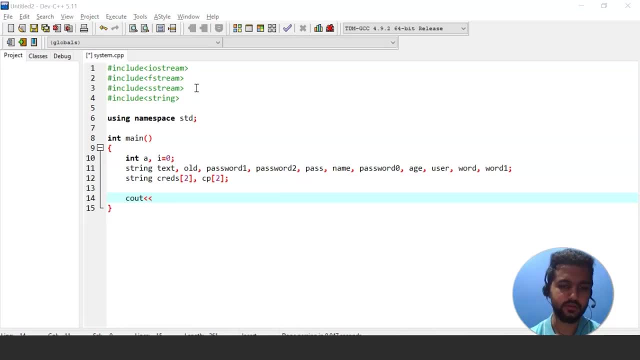 All right, Display and interface. and in that interface we will show four options like register, login, change password and end program. So let's just do that, All right. So let's name it security system And then All right. 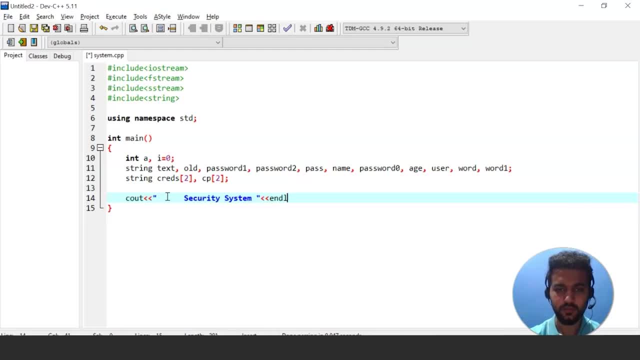 So all right, So let's do that. And then All right, So, as we are creating interface, so let's make it look good, like we can do some things like that, and I'll put extra space now. here we can do one thing like, can do like this: 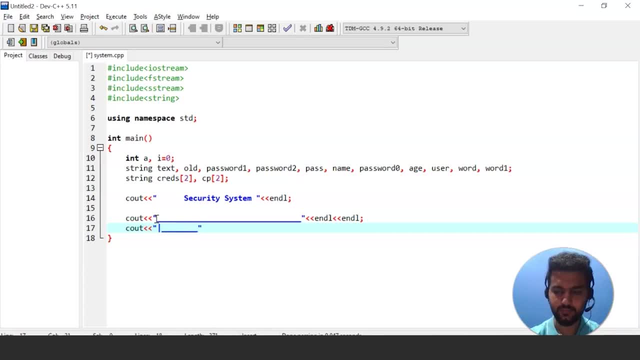 it's up to you how you want to beautify your interface. that's all upon you. so I'm basically doing that register. Similarly we will do for others that we can just copy paste. it will save our time. so basically, first would be register, second would be login and third would be change password. 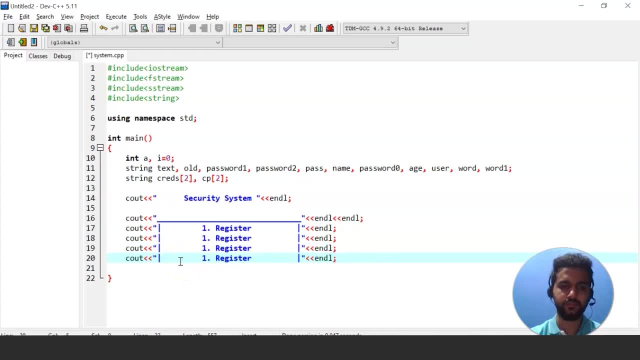 and four would be login. Next would be end program and we can do one more thing. all right, now let's make it to. this would be login, key would be change password, old. Fourth would be end program. All right, so register login, change password and end program. 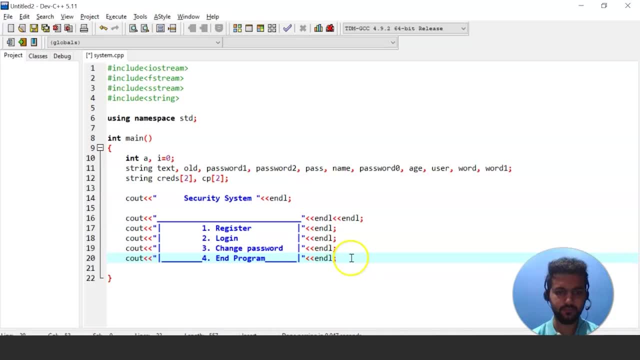 So we have created four of these. So we have created the four choices. now, after this, we will be asking the user to enter any choice, like if you want to register, login or change password Or end the program, so he can select one, two, three or four. for that we have to take an 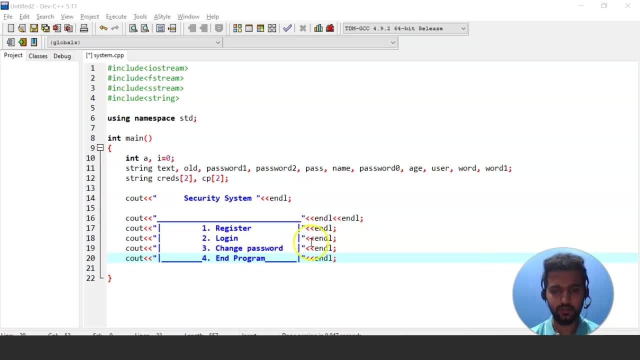 input from the user. So we will do that. First of all, to add some space, we can do ndel all right. So now we will use a do while loop. So inside the do we will again use ndel Right, so that there would be some difference between this register login interface and. 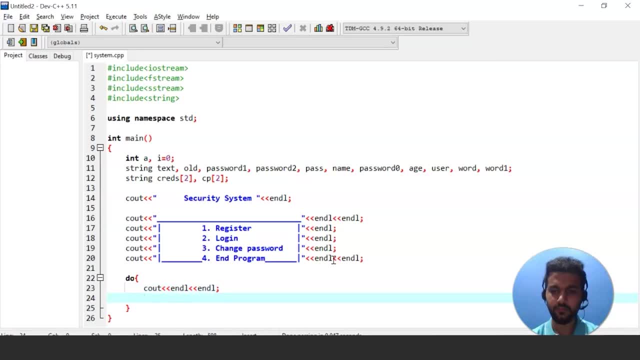 the choice that we will be asking right now. see out, and your choice. So here we are asking the user to enter one, two, three or four, as per his or her choice. All right, All right, All right. So see in, here we will be taking the input. let's say a is the input. now we'll use a switch. 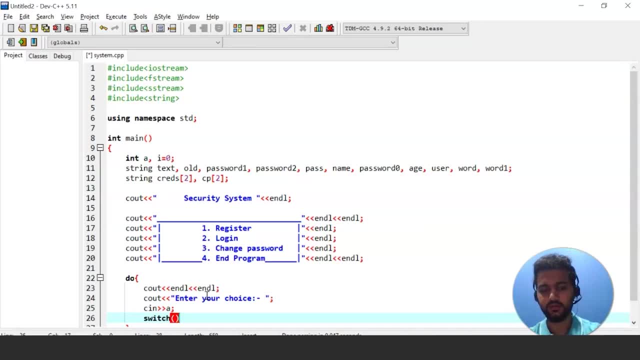 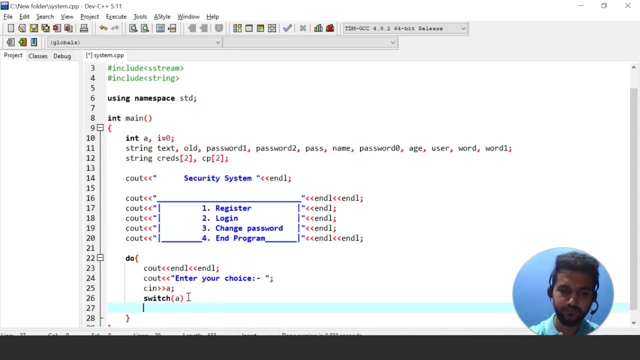 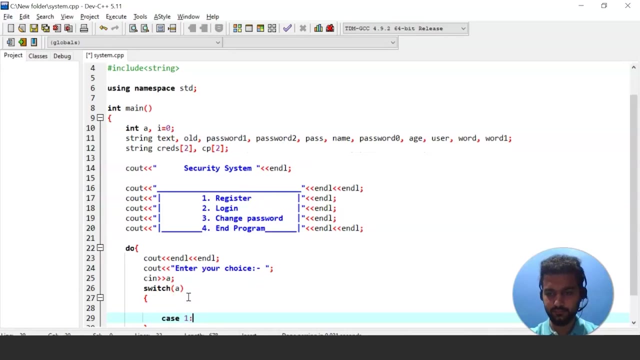 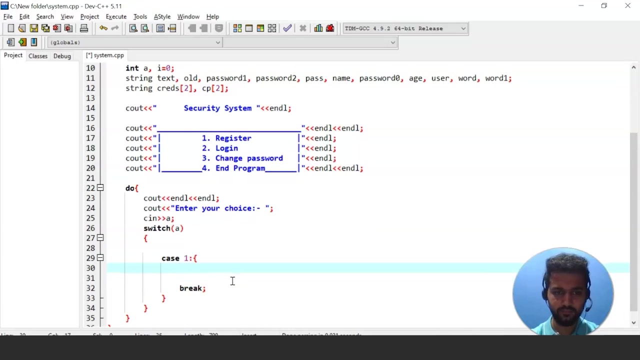 case right switch and inside the choice that the user will enter. All right Now. Okay, So this one would be the first of all case one and inside case one. let's go a little bit, All right. So inside case one, first of all, we will be printing something like register as as the. 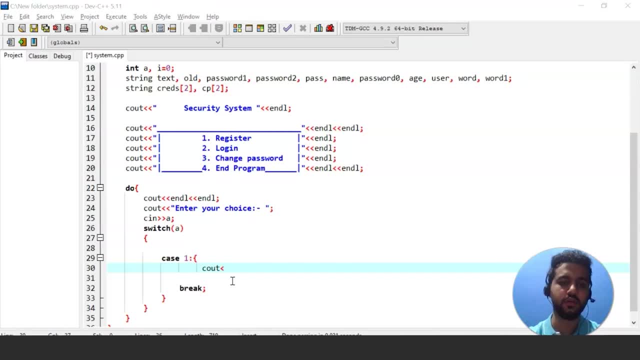 user has best one, So he won't register first of all. So we'll create an interface over here as well. So let's do that. Okay, See out. Okay, All right, Let's do it So, like we previously did. 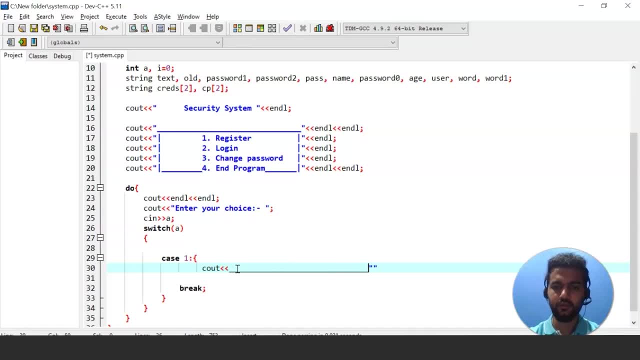 It's your choice, Like how you want to do it right now, We can All right, All right, register and l alright. after that, again, let's leave some space here, or we can do it above as well, like here also, we can do this. 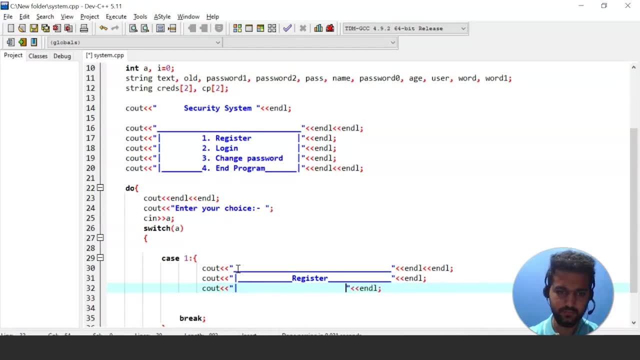 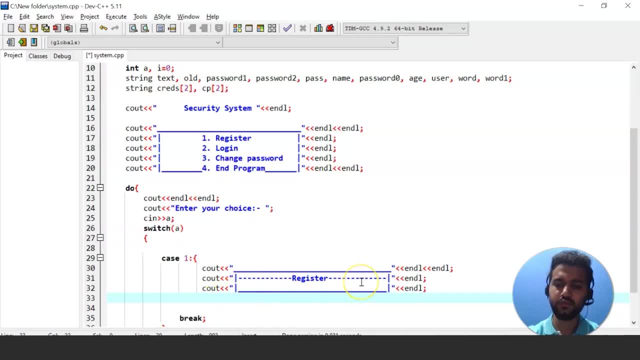 all right, so register here. we have created now we'll use to Wendell. because created now, we'll use to Wendell. because created now, we'll use to Wendell. because we want to create some gap in between. we want to create some gap in between. we want to create some gap in between- enter your choice and this interface. 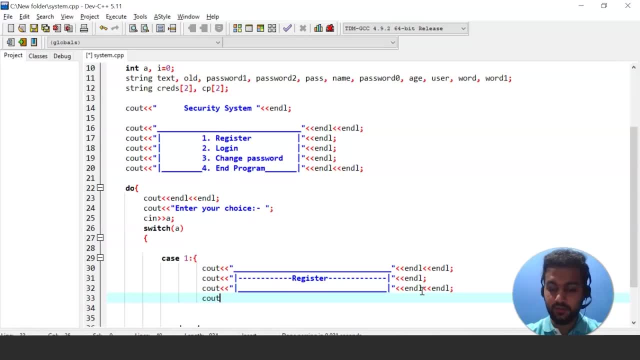 enter your choice and this interface. enter your choice and this interface: so right, so we'll print a message. enter. so right, so we'll print a message. enter. so right, so we'll print a message. enter your username. it's like: please enter your username. it's like: please enter. 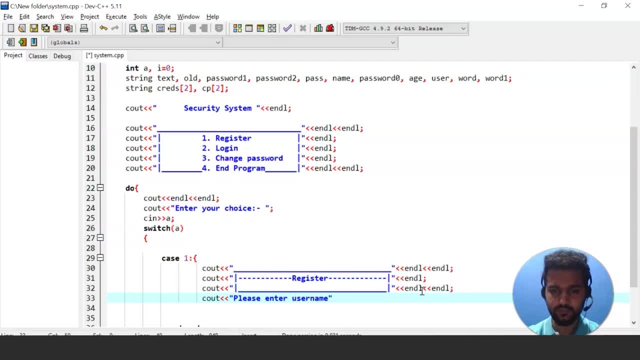 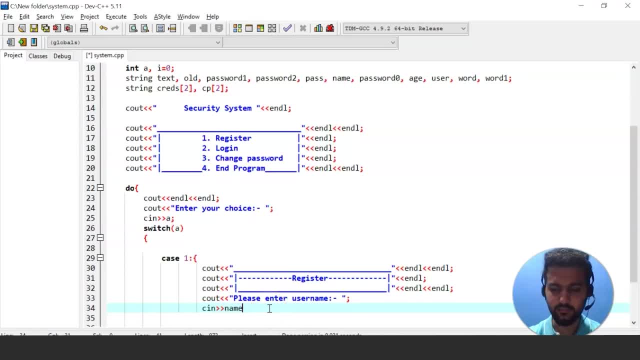 username. so we'll take the input of that username. so we'll take the input of that. so here we will write name. all right now. so here we will write name. all right now. so here we will write name. all right now. the user will have to enter password. 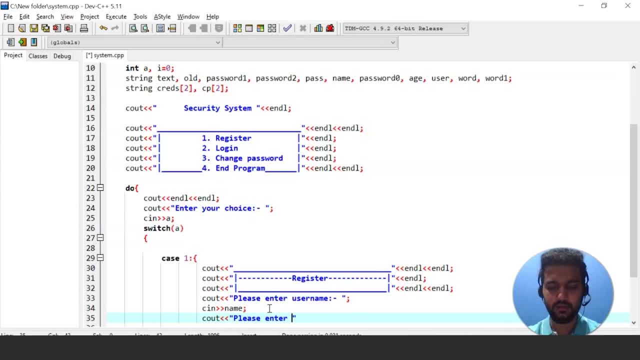 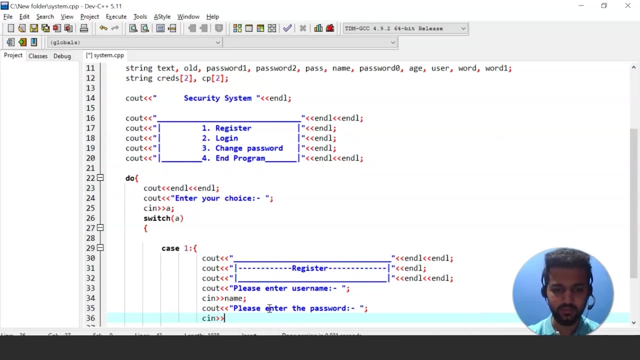 the user will have to enter password. the user will have to enter password also. so right, please enter the password also. so right, please enter the password also. so right, please enter the password. so after this, the user will enter the. so, after this, the user will enter the password. so we will be taking the input. 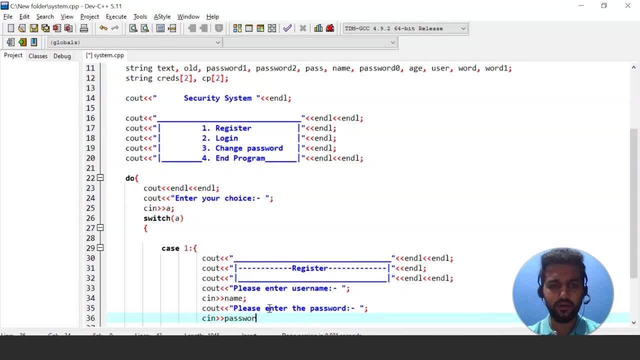 so after this, the user will enter the password. so we will be taking the input. so after this, the user will enter the password, so we will be taking the input of that. so we have already created of that. so we have already created of that. so we have already created these variables. as you can see, name we have. 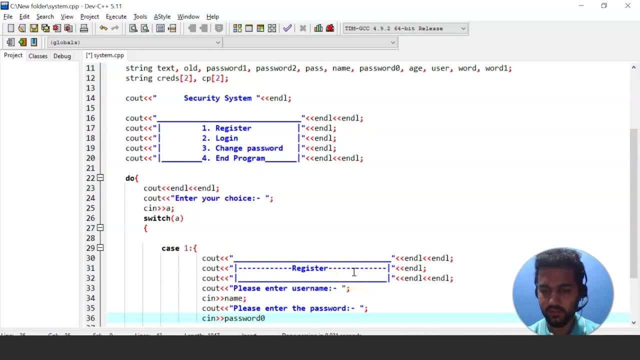 these variables, as you can see name: we have these variables: as you can see name: we have created. and password 0 also we have created, and password 0 also we have created, and password 0 also we have created. so we'll use that password 0 all. 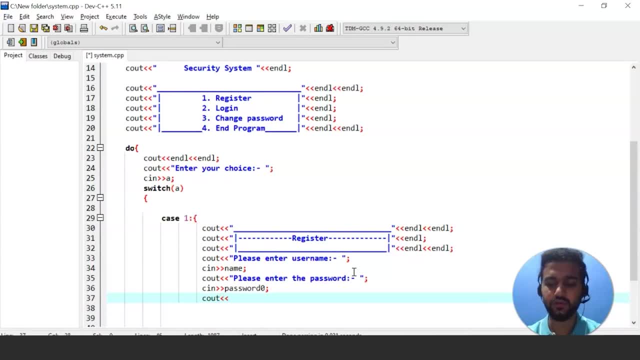 created, so we'll use that password 0. all created, so we'll use that password 0. all, right now. we'll ask the user to enter. right now. we'll ask the user to enter his or her age, so we like. please enter your age and whatever credentials you want them to enter. 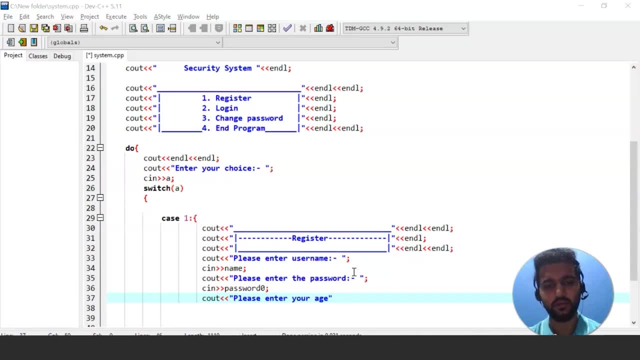 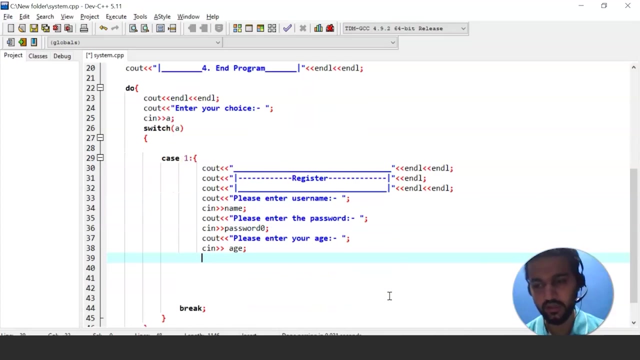 you can do that. you can also take the input of the address or something personal that you want to store. you can also do that, so all right. so please enter your age in age. all right, this name, password, 0 and age. we have already created these variables. we have initialized these variables. 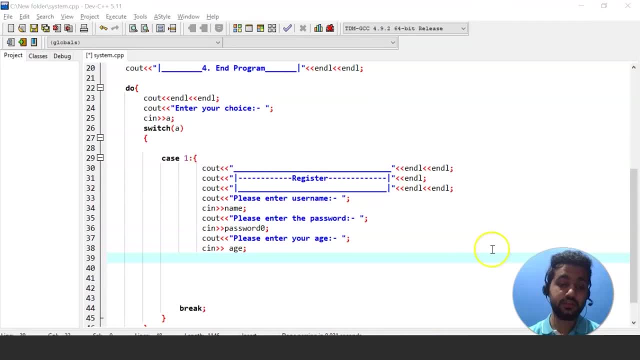 alright now. now we will store these details- that is now name, password, 0 and and age- into some file, and for that we have to use the file handling operations. so we'll use those like. we will create off stream class. we will create an object of off stream of one. 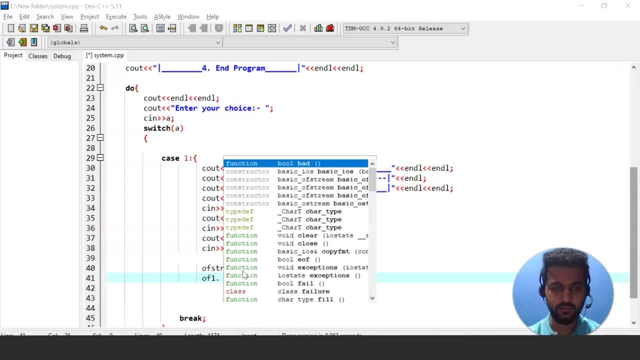 and of one, so we will use of one, as it is the object of off stream class. and why we have used the off stream class? because it is used to open a file to write something in it. so here we want to store name, password, age in that file. so basically we have to use off stream only. 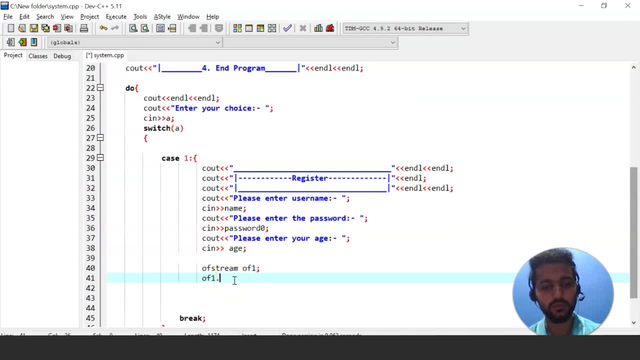 and if stream class is used when we want to open a file for reading purpose. but now we want to open the file for writing purpose, so that because of that we have used off stream class. so here we will write of1. that is the object of our stream class dot open. so 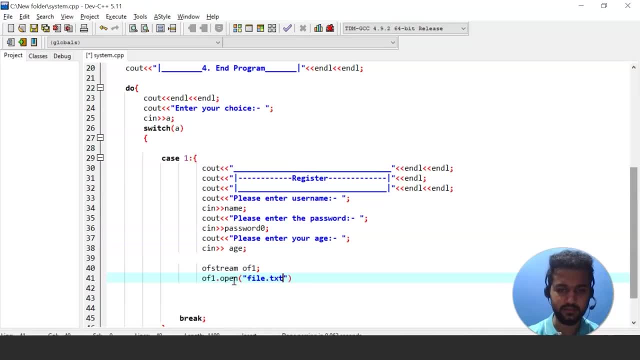 inside this we will write the name like that: file: dot. txt. it will open the file. all right. now inside the if block we'll write of1 dot is open, underscore open. this is a function. all right, we have. one dot is open. it will keep on moving till. 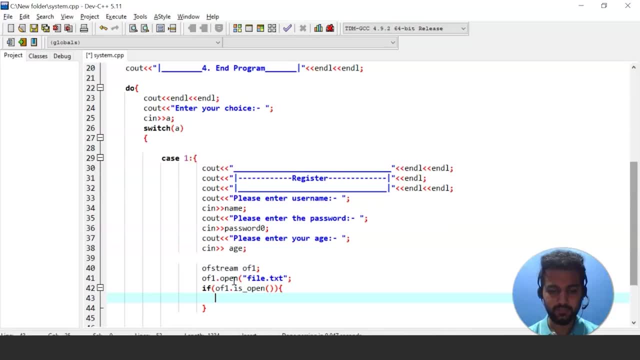 all the details will be entered in the file, so we'll write of1. so here, basically, we are writing the details inside the file. we'll use slash in because we want the username and password in different lines, so that is why we have used slash in here. all right, oh, f1 password. all right, password zero. it was sorry. 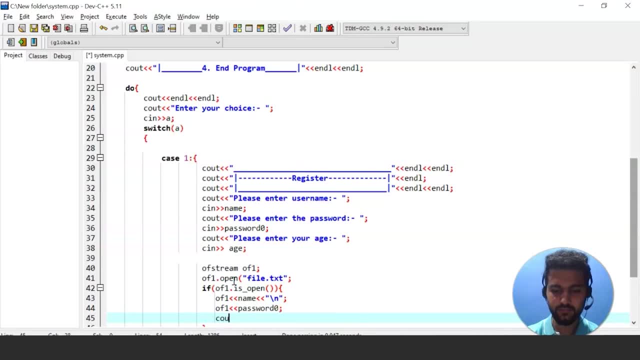 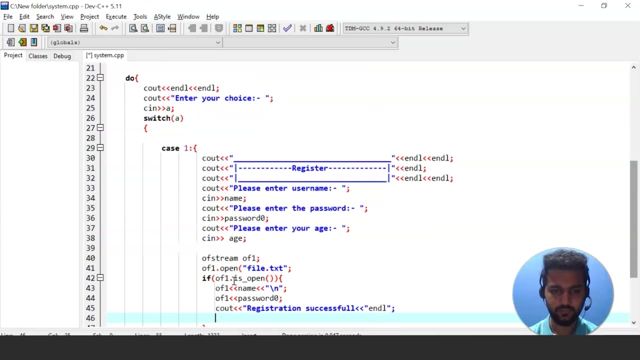 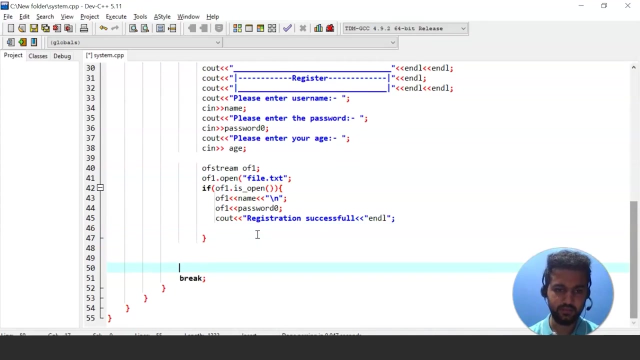 now we have stored the name and password. only it is time at development, so we got our Inte. now we'll write registration successful. all right, registration successful is done in this case. here we have taken the input of username, password, age and stored all these details in the file so that we can use it later. now. this was the case. one registration is done. 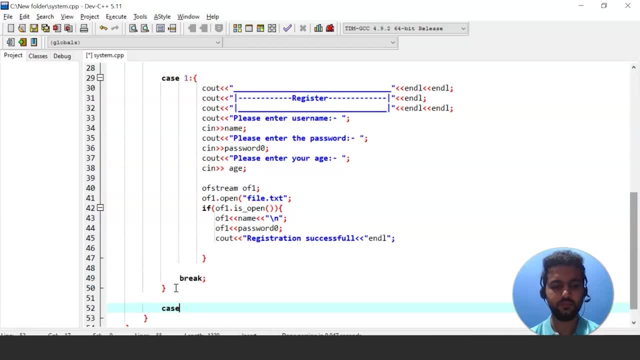 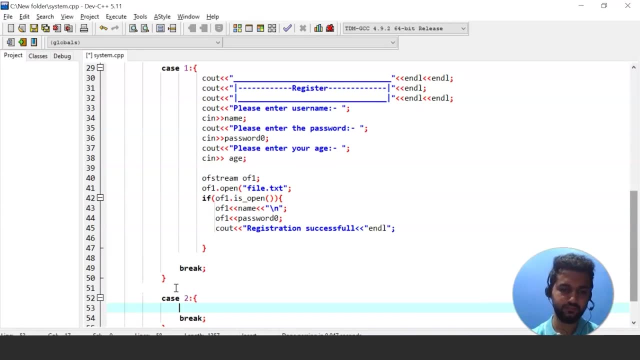 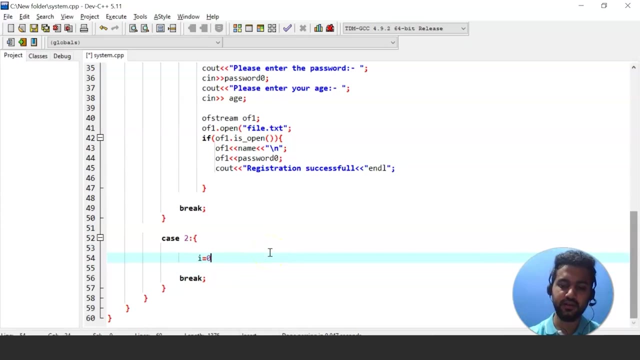 in case one. now we can move on to case two. similarly, we will create a case two now inside this case two, all right now, inside this case two. first of all, we'll initialize I with zero why we are doing this. I'll explain that later. so, similarly, we will create the interface that. 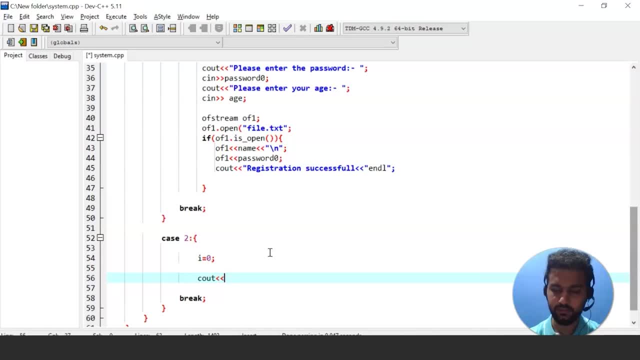 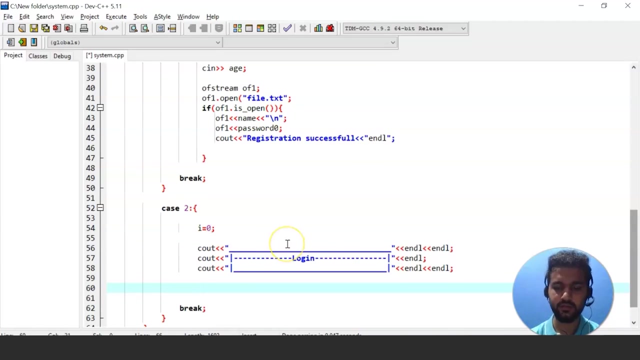 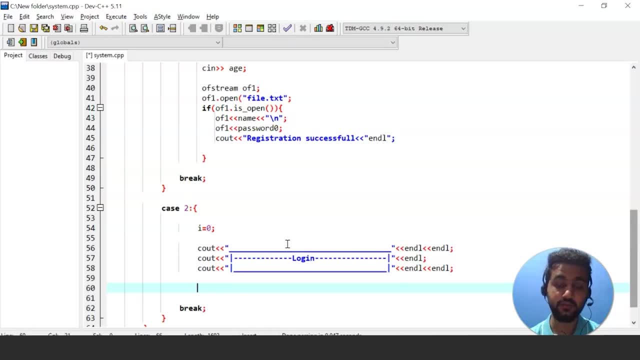 so, as i previously told that if stream is used to read from files, open and read from files. so we'll create if stream class and object if stream, if1 or let's say of of2. so this is the object of if stream class. now, using this object, we will open the file of2 dot open. 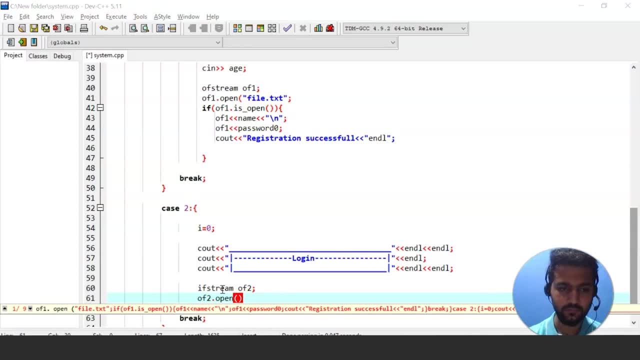 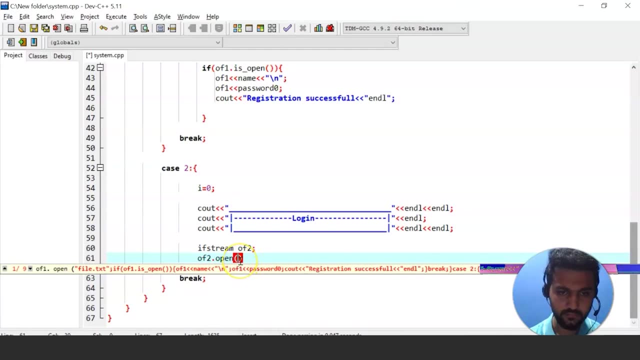 now of sorry. here we'll write file dot txt, all right. So here we have opened this file and now we'll take the input. like we'll have to match it whether it is the same person or not. So we'll take them. input will write: please enter the user. 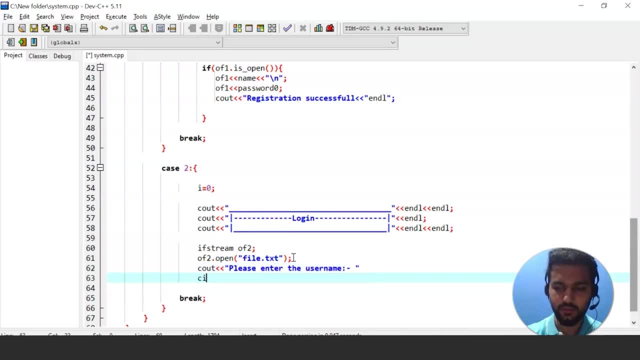 name. see in user the other variable that we have created now. see out. please enter the password. All right, So it also will take the input from the user, will write the other variable. that is pass. That's why we have created so many variables. 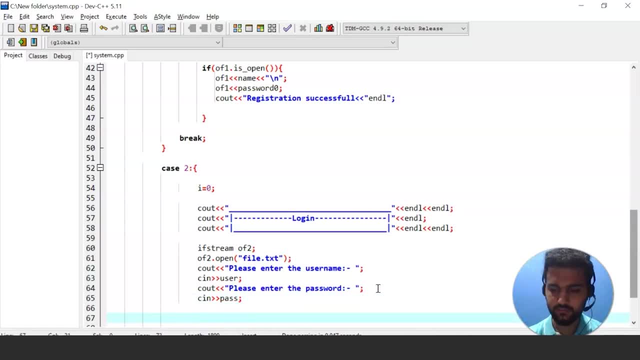 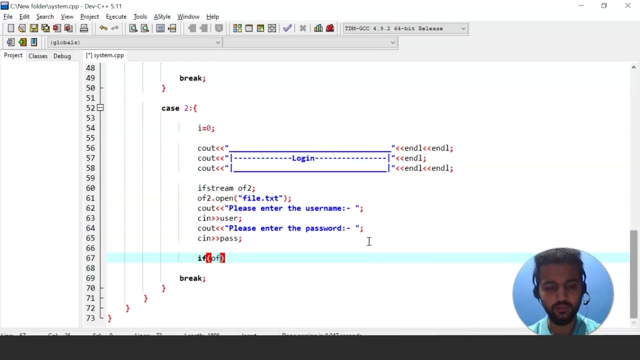 All right, No, No, Let's roll it a bit. No, If, similarly that we have done previously, of two dot is underscore open, It will check all the files. basically is open, then here we will use a while loop: Note who F to not end of file. 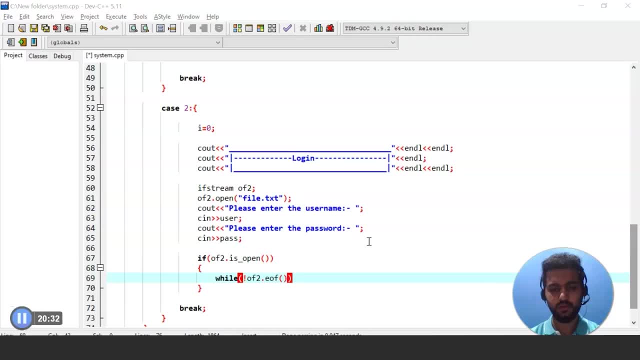 So here We are using the end-of-file function. from this EOF or end-of-file function, We can detect when the end-of-file is reached. it returns non-zero when the end-of-file has been reached, otherwise it will turn zero All right inside it. 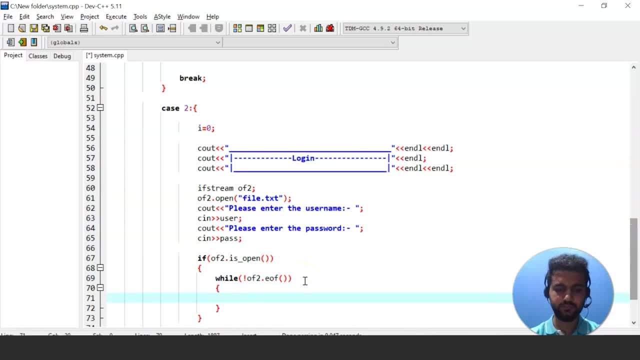 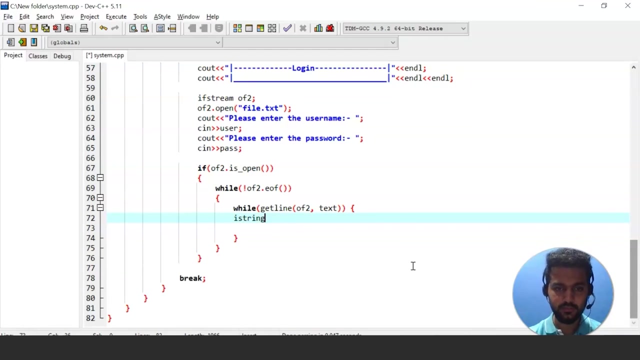 Now we will create another while loop, While get line. who have to? that is the object And text. that is a variable, All right. No, inside it We will write I string Stream I s s Text, All right. 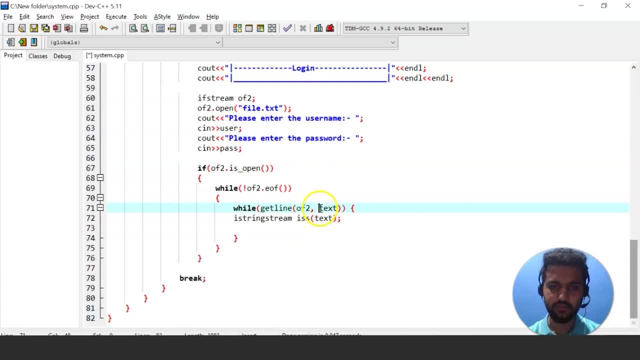 Now I'll explain the part. So here in this part, get line part- So a while loop together with the get line function is used here to read the file line by line. So using this, the get line function, the file will be read line by line. and this I string stream object. 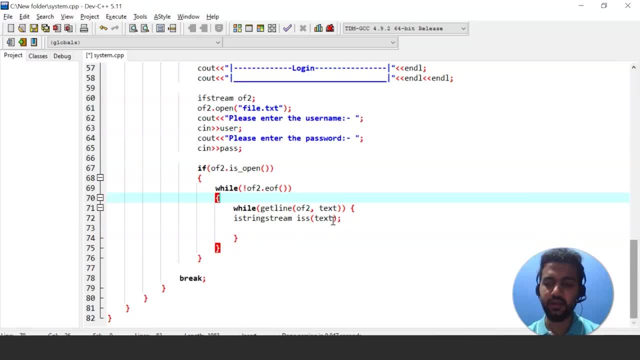 So I string stream object is used to stream the string and store it using the extraction operator. After this we will be using an extraction operator where we will store The string. All right, Here we have used extraction operator and here we are storing. 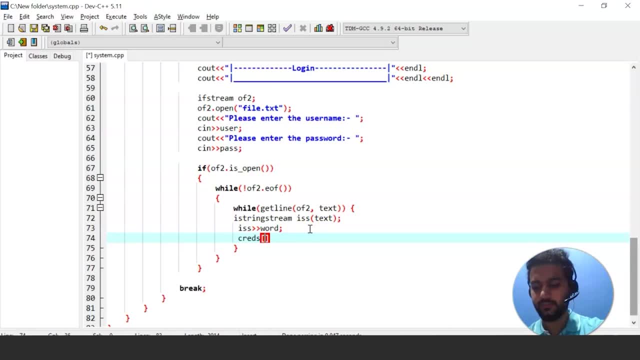 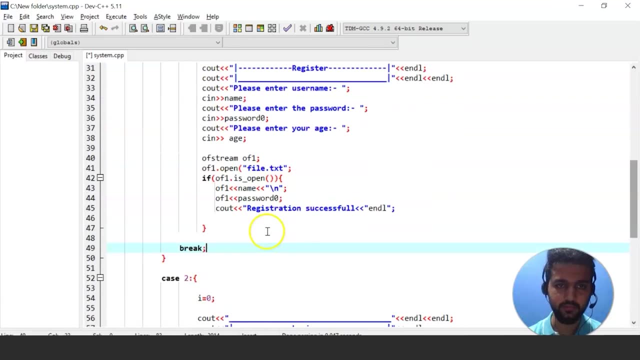 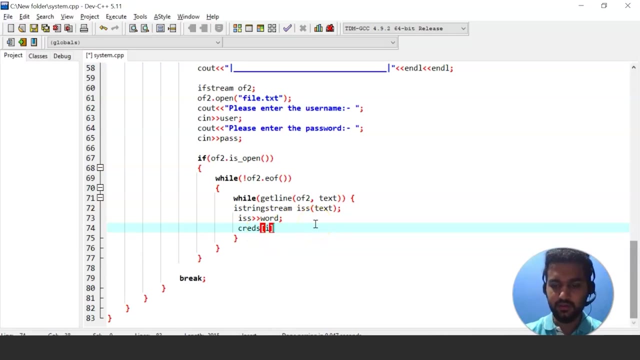 Now in the creds array that we have created We will be using Here. we were All right. So in creds array We have already declared this. We will store the word first of all, And then we will increment because one by one. 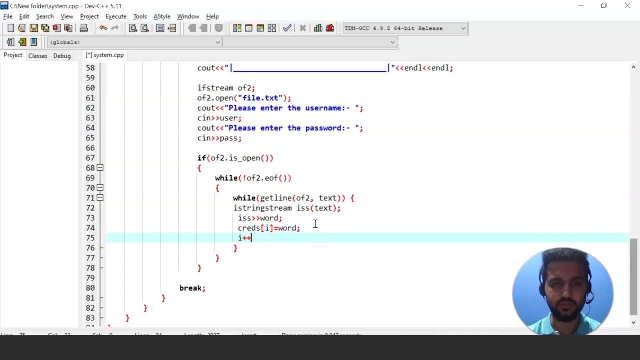 The in the zero position. first of all, first username will be stored. then the password will be stored in the second position, So we need to increment that. All right? No, We will match if the registered username matches with this username or not, And similarly we will do for password. 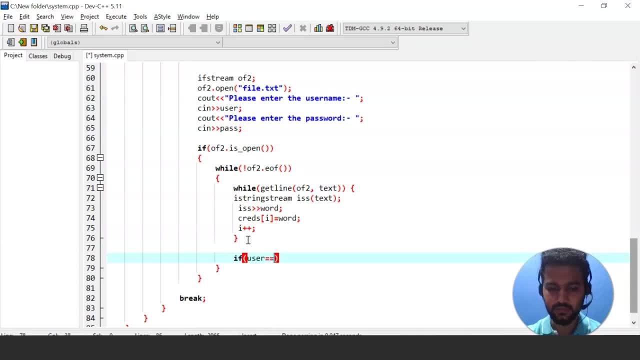 So we can do like if user equals to credits at the 0th position, that is the username, username the user has entered first, So it must be at the 0th position and the password would be at the first position and index one. So for that we can use: password equals to. 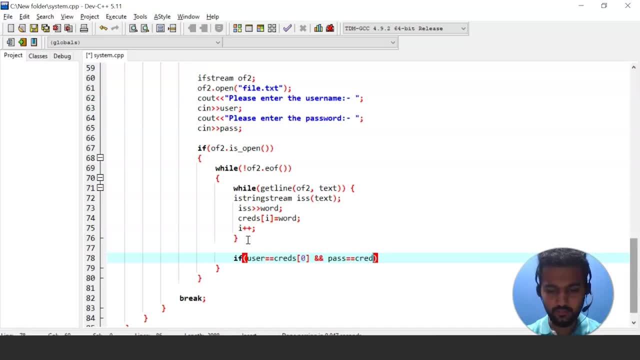 Creds at Index one, Then We can print a message Saying that login Successful, All right, No To add some space we can use. and Now, after displaying this login successful sign, We can print the details like We can write: 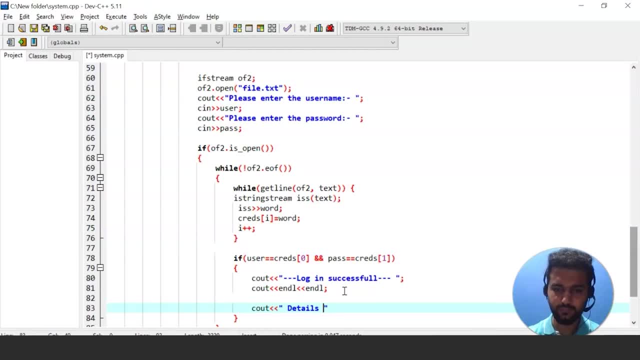 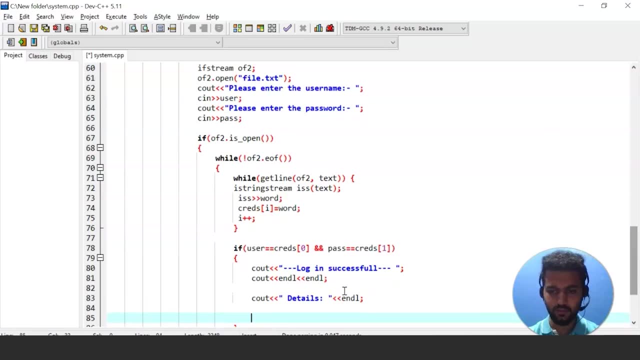 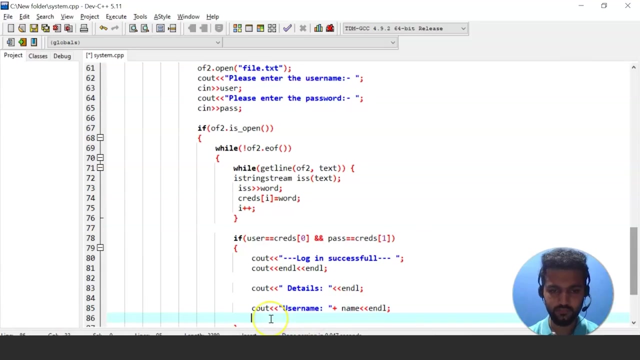 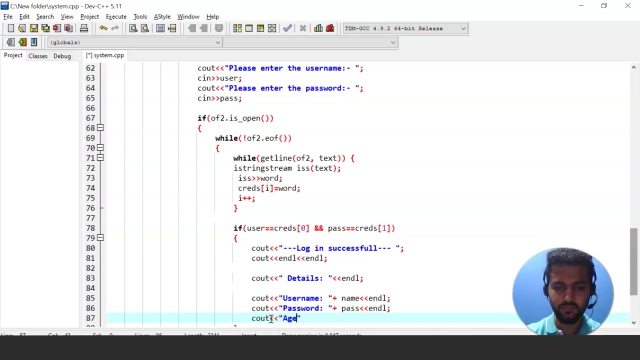 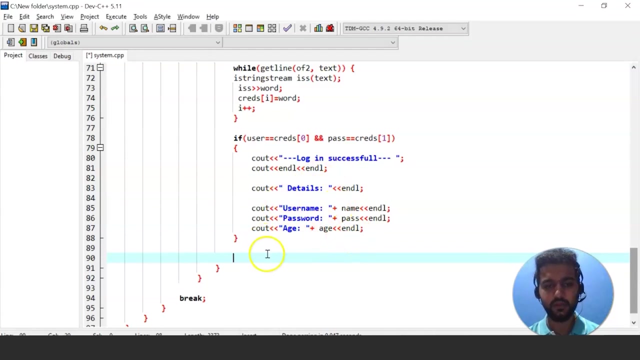 Details. We can write: See out Username Username: All right. Similarly for the password will do So, Also the Good. so here we will show the username password, age details to the user now in the else block. so where the password and login. 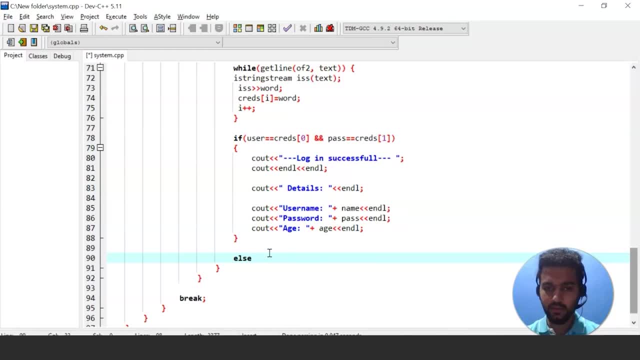 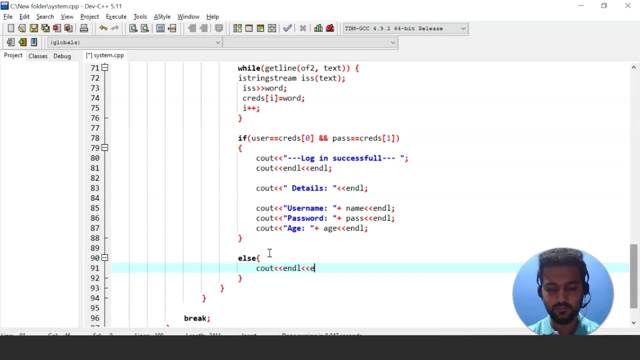 credentials will not match. in that case, now we will do so. for that case, we will write first of all: let's create some distance so that it looks nice, alright. so first of all we will write incorrect credentials, alright, incorrect credentials. after that we can do one more thing. 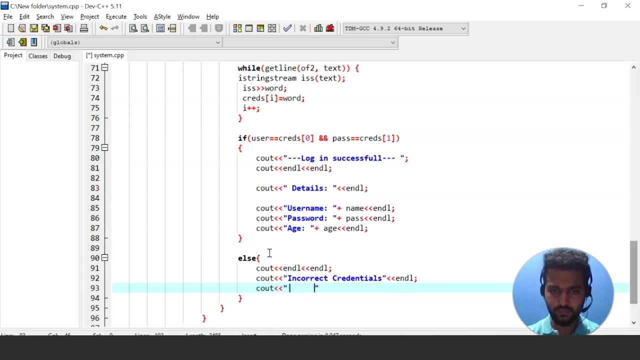 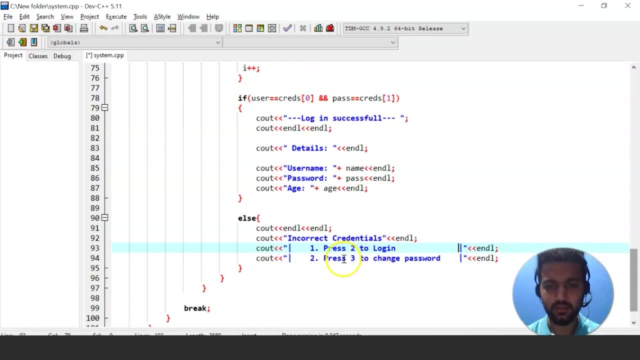 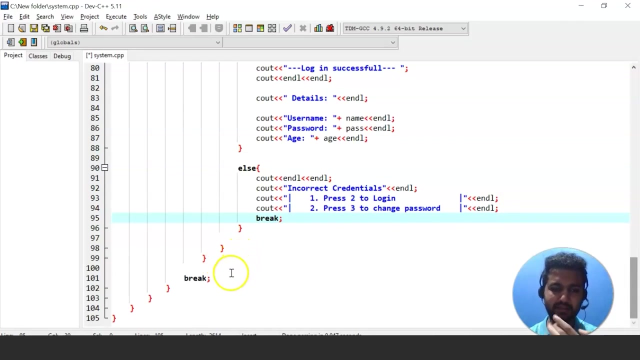 so here we go. so if the details are incorrect, so the user can login again, try, or he or she can try to change the password. now we will add the break statement also here. we have added the break statement. now, as you can see, our case 3 is also done. so what we have done in case 3 is: 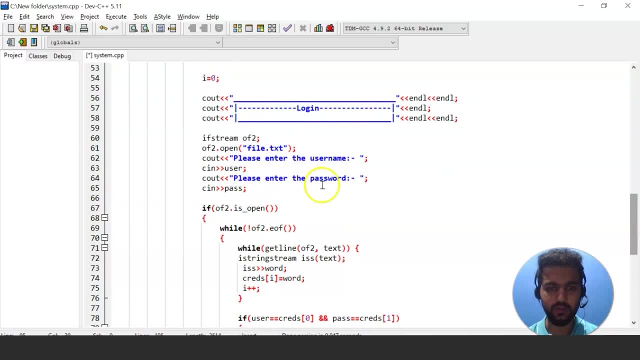 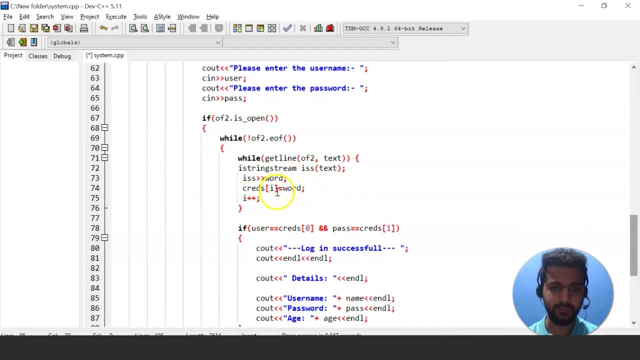 like, we have taken the input of username and password and then we tried to store it at credentials. that is an array. so at credentials 0th position, that is, index 0, the username will be stored and at credential first index, the password will be stored. then we will try to match the username that the user has entered while 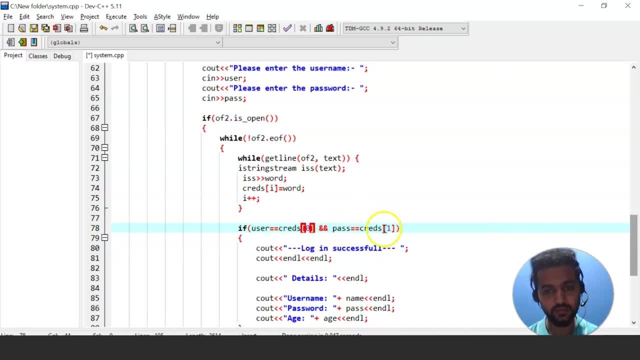 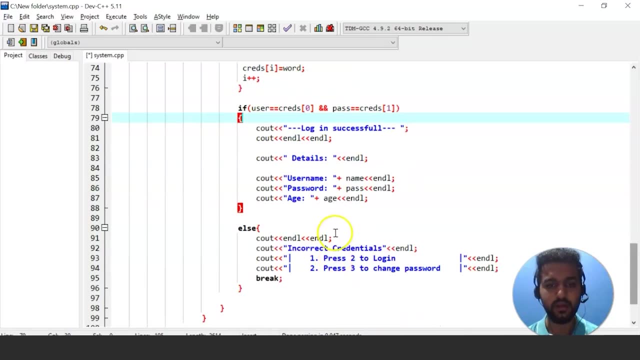 registering with the credits at 0th position and password with the password. so if it matches, the login will be successful and the details will be shown. and if the details are not matched then it will show an error- incorrect credentials- and press 2 to login and press 3 to change password. so 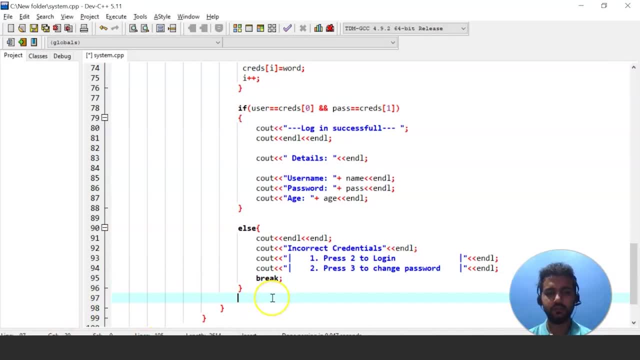 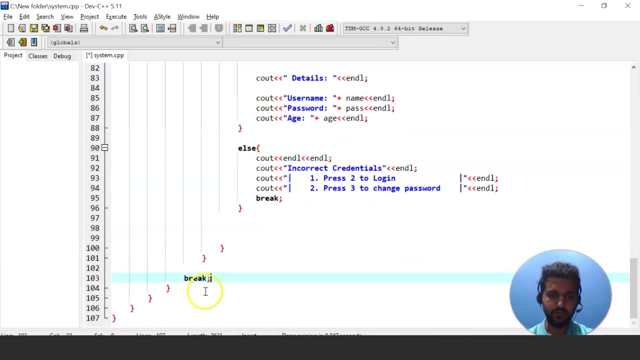 this was the case 2. now let's move on to case 3. from here we will create the case 3. alright, now in case 3 we will write again. we will first of all initialize i with 0. now here let's scroll it a bit. 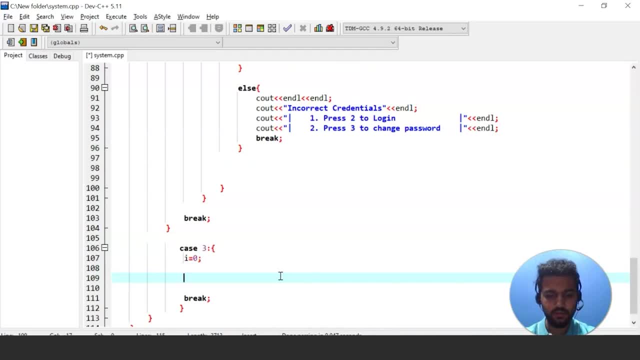 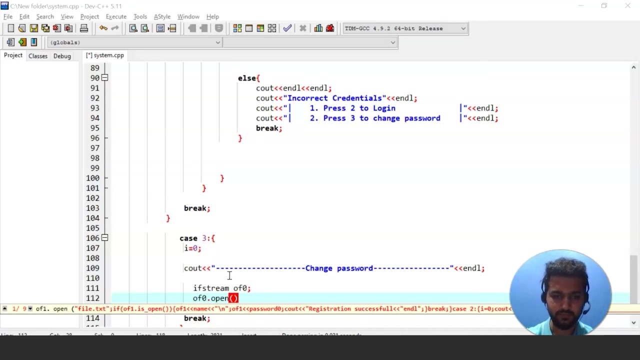 ok, yeah, so here we can write like change password. so let's do this: change password. so now, after displaying this again, we will open the file using that. if stream here, if stream of zero, now using this object of zero will open the file dot txt. file dot txt. 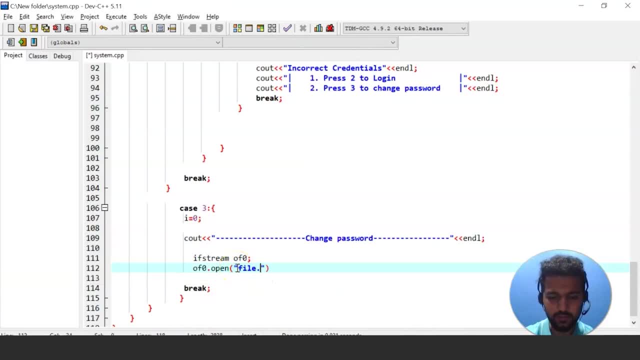 all right. so here we will write file dot txt. after opening this file we will display a message to enter the old password. so because we are changing the password, so first of all we'll ask them to enter the old password. so enter the old password. now we'll take the input bold. this is the variable. 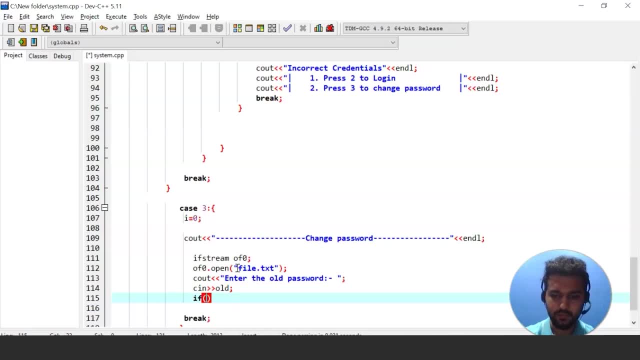 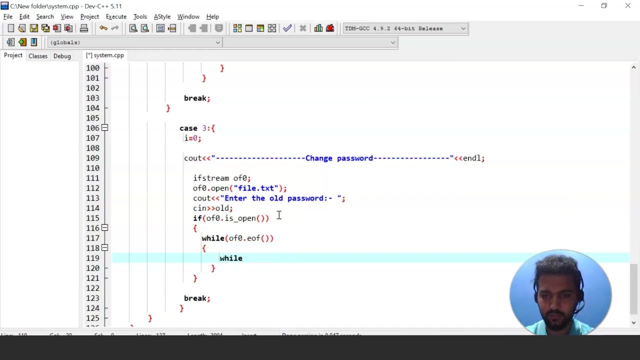 now we'll use an if condition that, similar to that that we have previously used, of zero dot is open, this file will remain open. now again, we'll use end of operation. function is underscore. end of file. right now, inside this while loop again, second while loop will be used, similarly that we have. 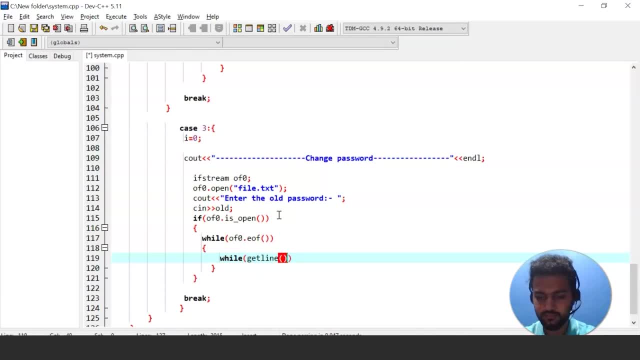 done previously. get line function again right. i string stream, I assess text, I assess word one here. basically, we are storing the data in word one, then cp, another array. so we will store word1 at 0th position, then we will increment cp. by mistake we wrote co. 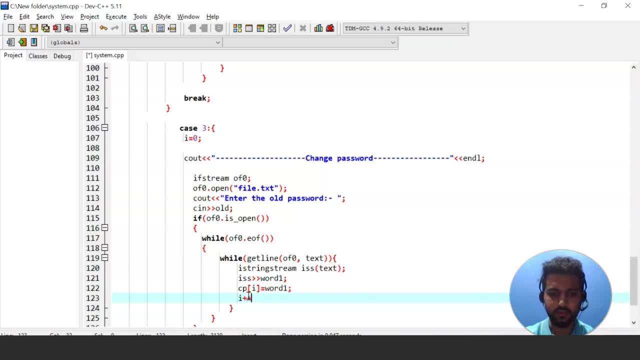 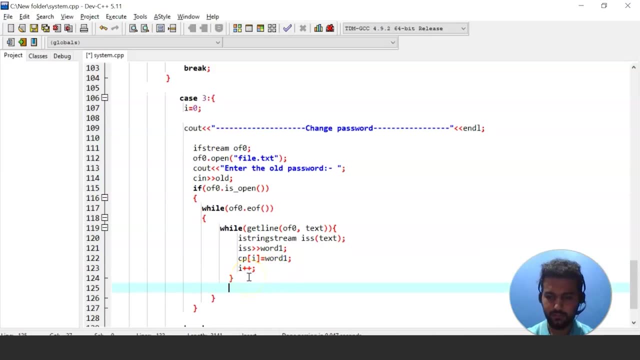 alright, now we will increment so that the password will also get stored. alright, now we will use if condition: if old password is equal to cp1. as we know, at cp0 the username is there, but we have to compare the password. so if old password is equal to cp1, that is. 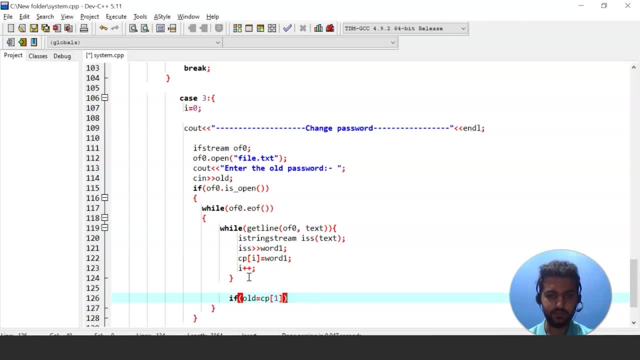 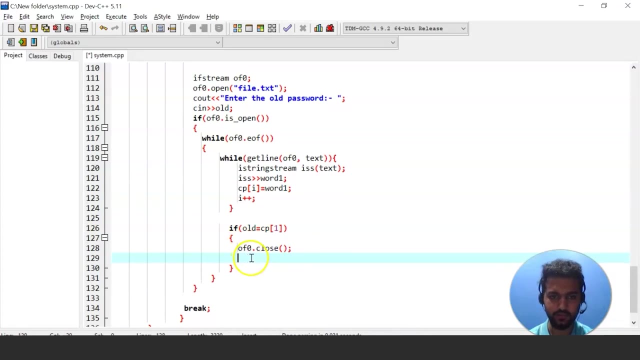 the new password that the user has entered, then, first of all, we will close the previous file to free up the memory space. alright, now we will open another file with offstream, object of1, because offstream is used when we want to write something, open and write, so. 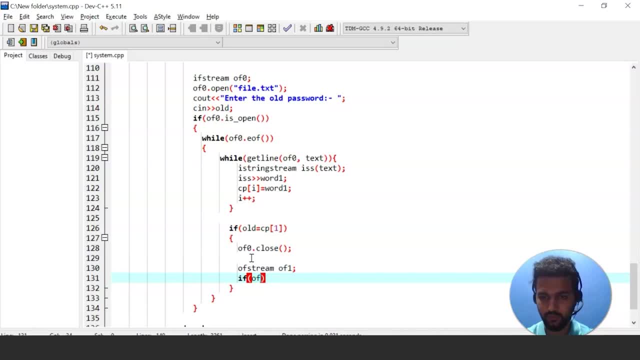 now we will use of1 object. dot is underscore open and now it is double actually. alright, now cout enter your new password. we are basically asking them to enter the new password. we will take the input of the password one. then we again display another message saying that: 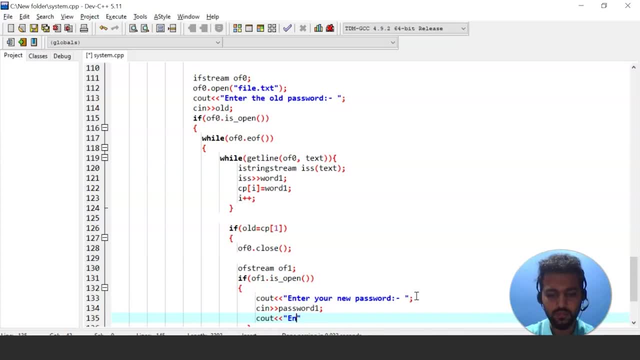 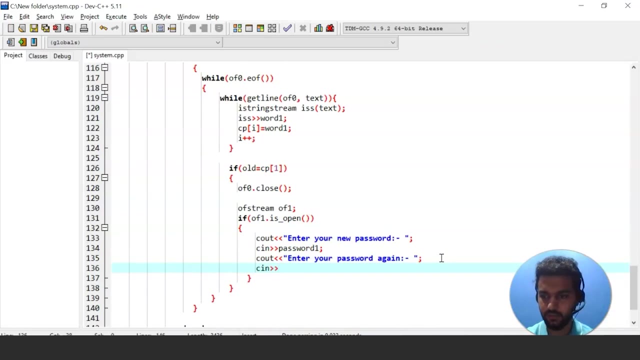 enter your password again. so enter your password again. again, we will take the input saying that password two. now, if password one equals to password two, password two- then we will overwrite cp, cp zero. that is, we are storing the zeroth index of cp at of1. we will basically overwriting. 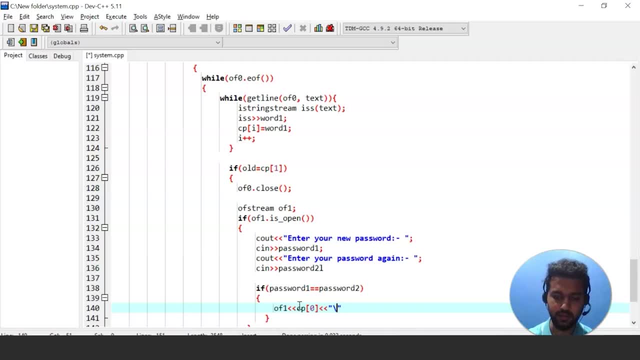 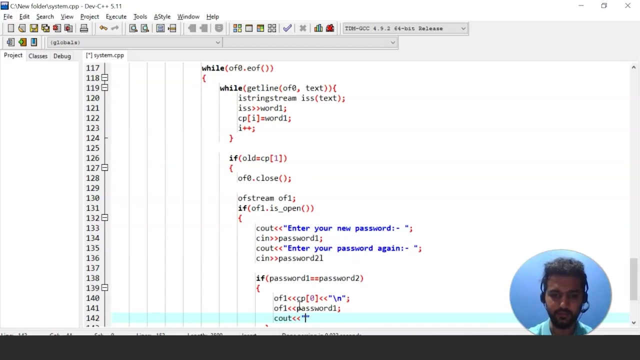 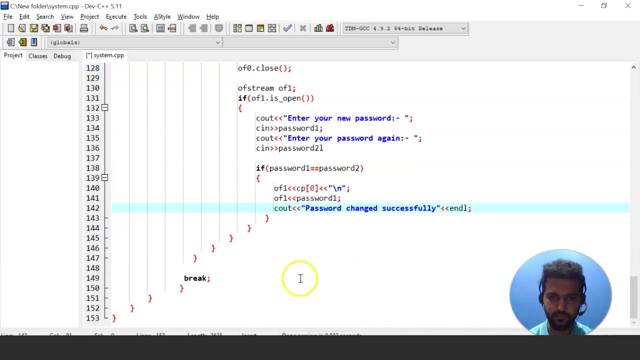 this slash and so that the username and the password displays in different lines in the file that is being created of1 password one. here we are basically overwriting now we will display the message after this: that password change successfully. alright, now in, else block, that is, if password one. 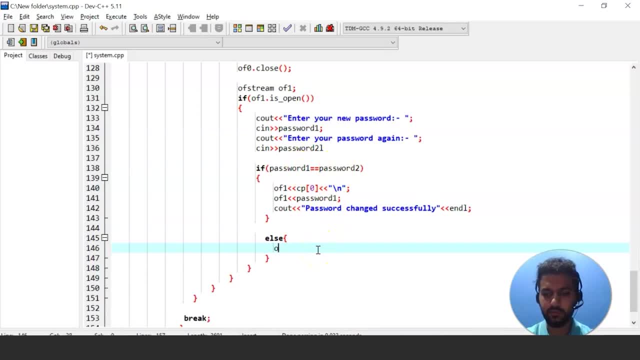 is not equal to password two. in that case, what we will be doing is of1. of2 cp, cp zero. after cp zero, we will again use slash n. alright, of1 old. that is the old password, so it doesn't get overwrite here. so now we will display: 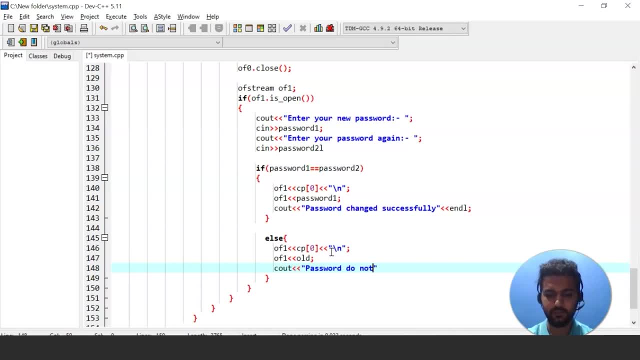 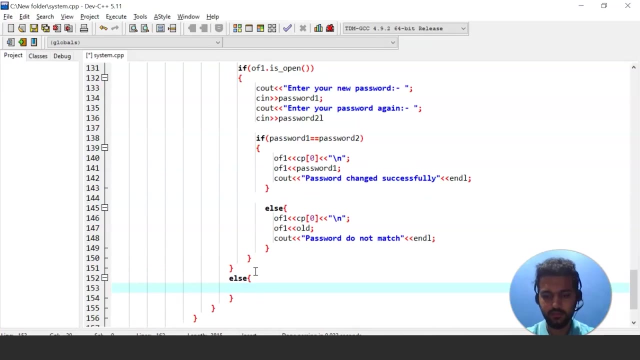 password do not match now for the previous. if we will create else condition in this, else we will print: please enter valid password. that is, if the old password entered by the user is wrong, please enter a valid password. alright, once this is done, we can use a break here. 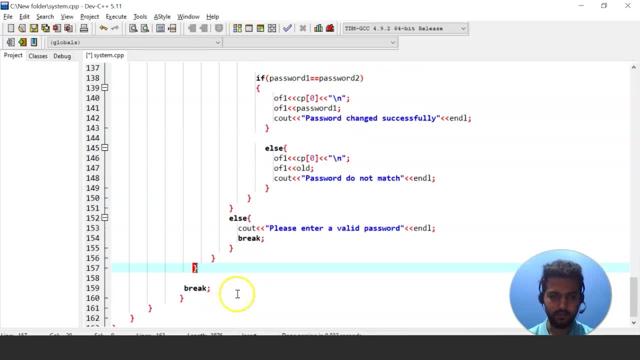 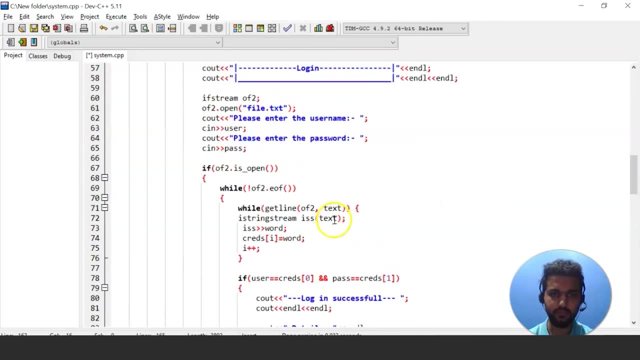 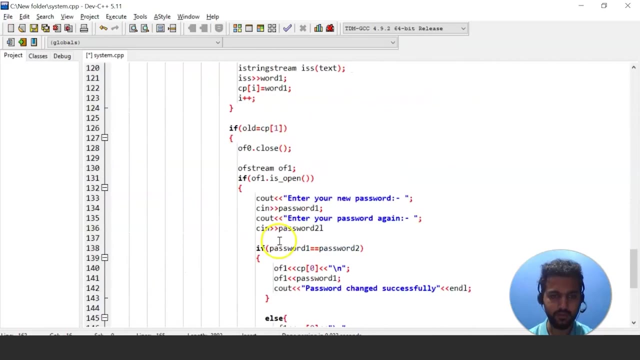 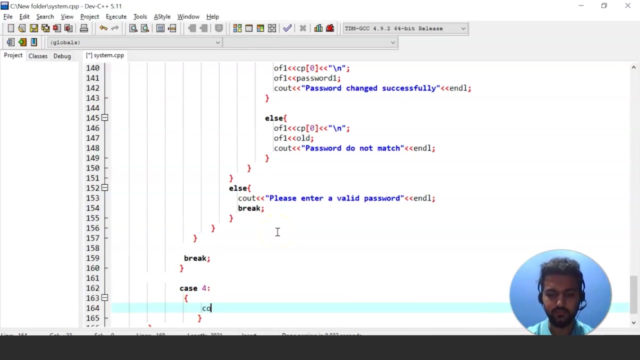 alright, now the break statement is already there. now, as we can see, there were four things like four options: login, change password and end program. fourth one is end program. now we will have to create case number four and inside that case we can do one thing, like we will just. 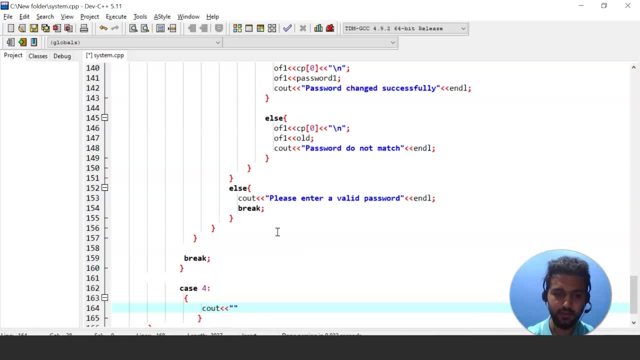 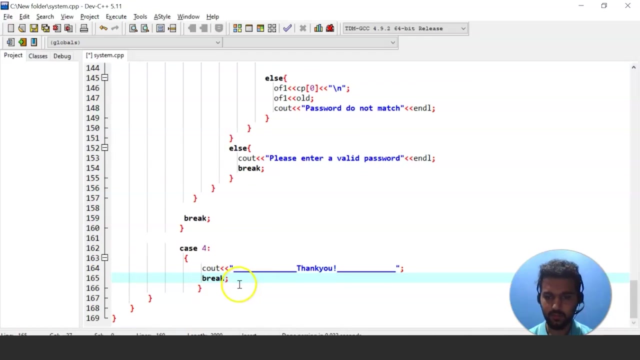 print one thing and use the break statement. we can write like: thank you, let it look nice. alright, so the fourth case is also done. now we can also create a default case. in the default case we can write like: enter a valid choice. like if the user by chance 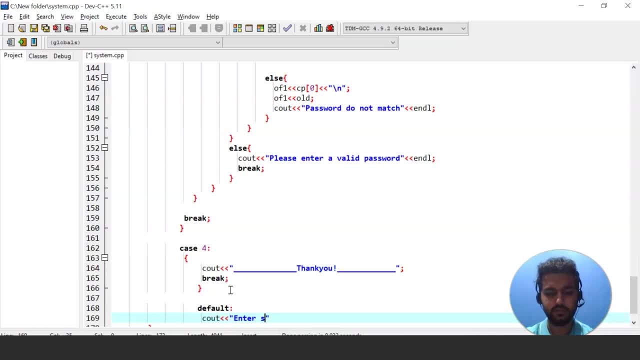 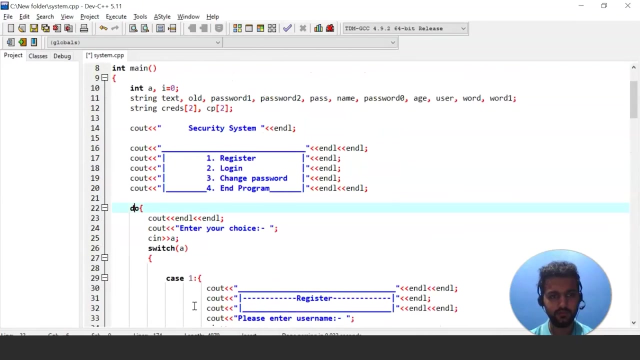 entered 567 other than 2434, then this message will be displayed. alright, now we will use a while loop. not equals to four. so so this is the while loop of this do do that we have created, as we can see this. do we have used the do while loop, so it. 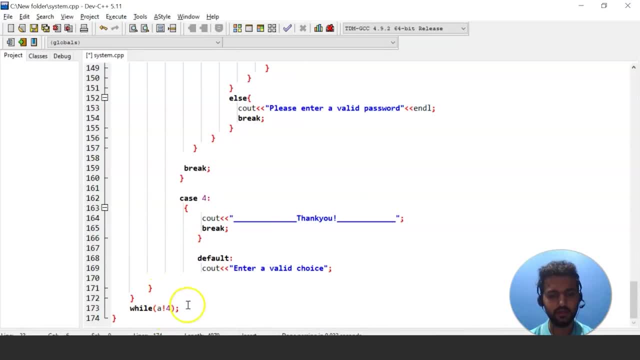 keeps on repeating until a- that is the choice- is not equal to four. once the user entered four, that is the end program. then it will not show the options. so that's why we have used this, while return zero. alright, our code is done. let's try to run this program. 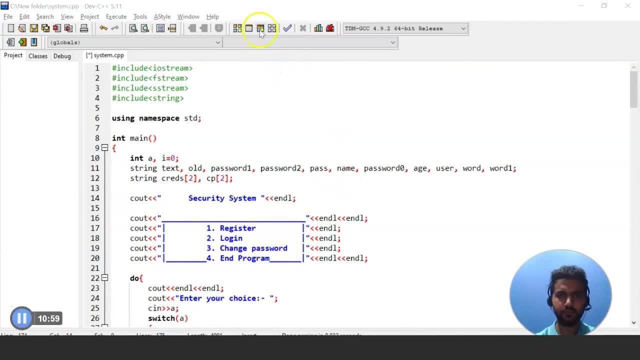 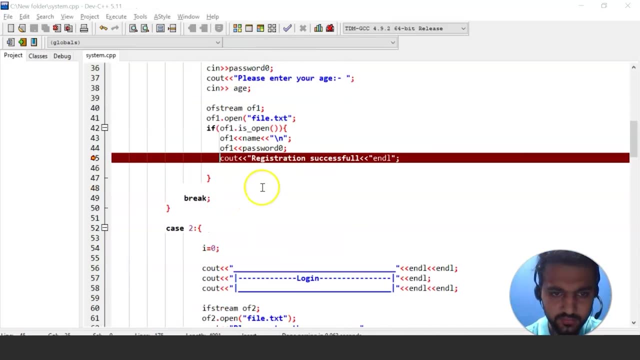 I believe some errors must be there. let's see. so it is showing some error over here. so we have used double quotes with and l, which we can't use. alright, now let's save this one, and now let's try to run this. we forgot to close this one. 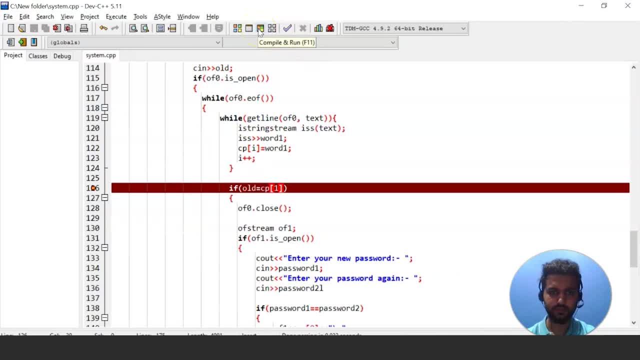 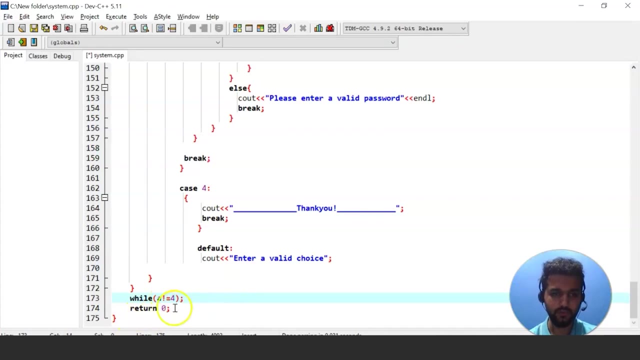 there must be some errors. there must be some errors again. so again, we will have to make it double equal to- and one more error is there, I figured that out- not equal to four. forgot to add equal to sign. now I am sure that, I am pretty sure that all the 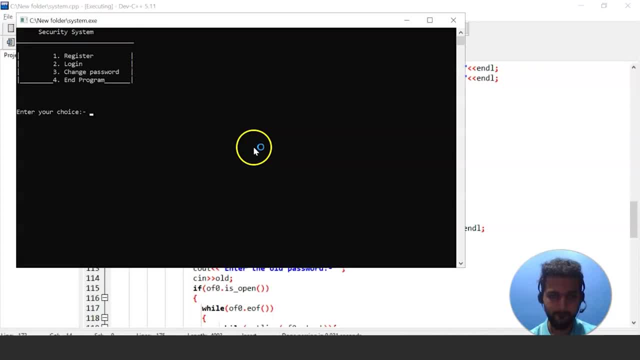 errors are resolved. let's try to run this again. alright, as we can see. one for register, two for login, three for change password, four for end program. alright, so first of all we will register. let's say we want to register. enter your choice one, let's say ak1. 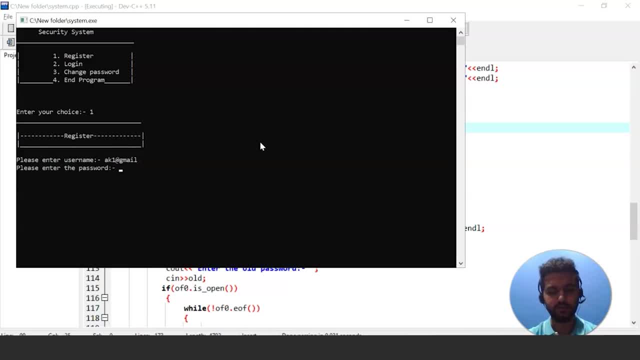 at the read gmail. so this is the user name. let's set the password. ak123 write age 24. registration successful. now we have to press two to login. again the user name we will have to enter. we will write ak1 at the read gmail. now the password. 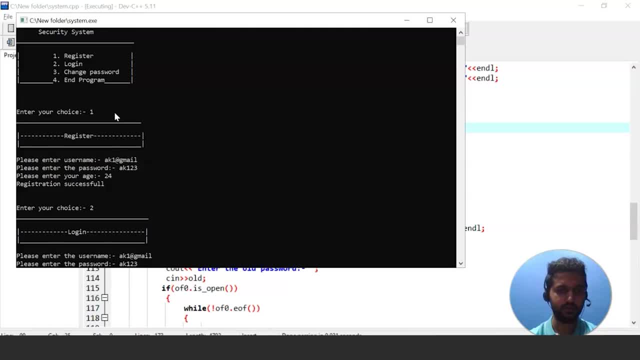 is ak123, as we know. so, as we can see, the details are here. user name is this, password is this and age is 24. now, let's say we want to change the password, we will click on three. as it is mentioned, to change the password we will have to click on three. 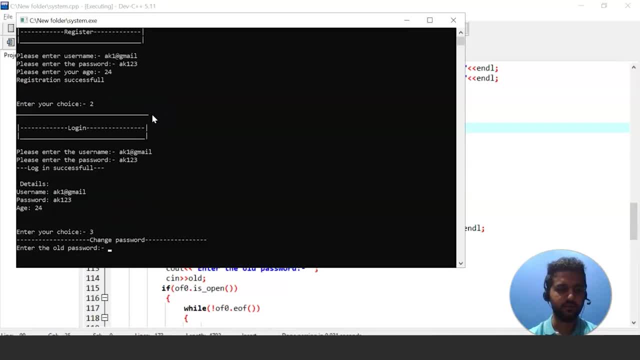 so we have clicked on three. so first we will have to enter the old password, which was ak123, now the new password, ak321, let's say. for the confirmation we will have to enter the password again, ak321, as we can see password changed successfully. now just to check. 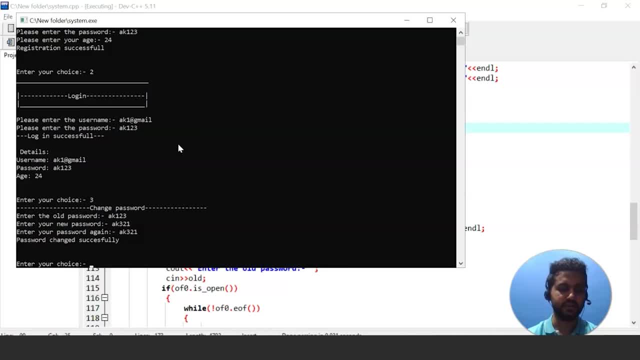 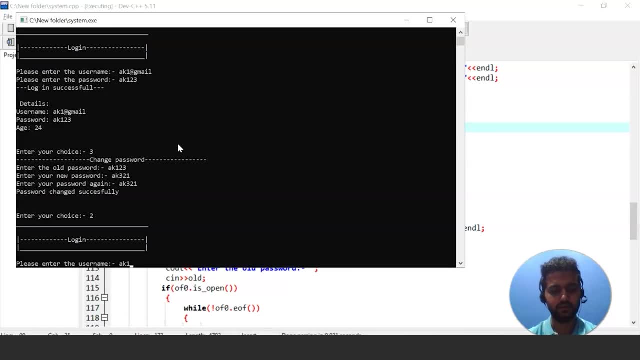 that if this password is really changed or not, we will login again. we will press two to login and enter the username ak1 at the read gmail and try to login with the new password, which is ak321. as we can see, the login is successful. username is: this password is: 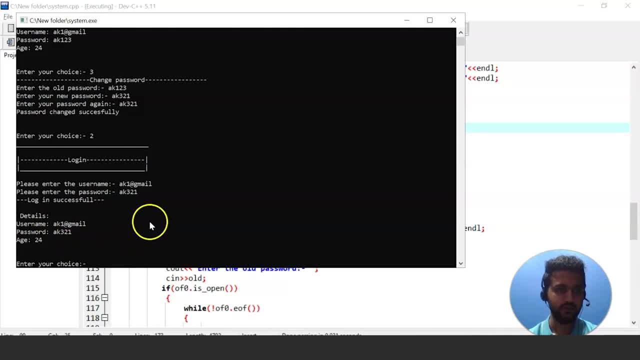 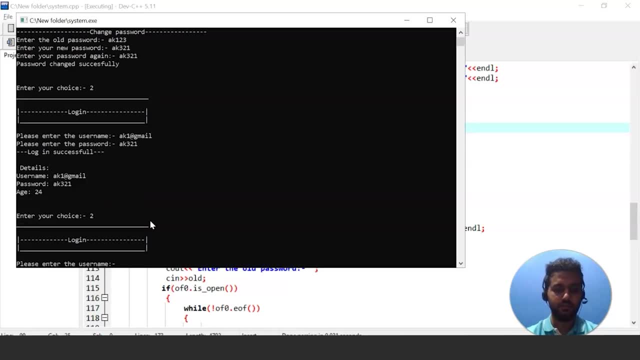 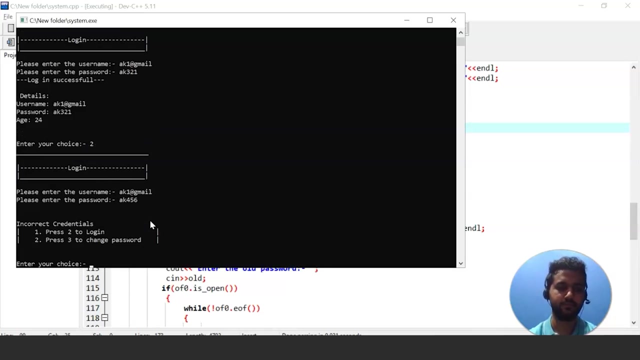 ak321321. age is 24. now, let's say, if we try to login with the password. so let's say ak1 at the read gmail: this was our username. now the password. let's say ak456. let's try to login with the wrong password, as we can see. 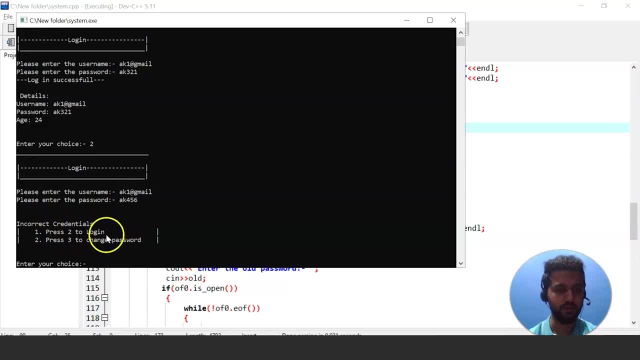 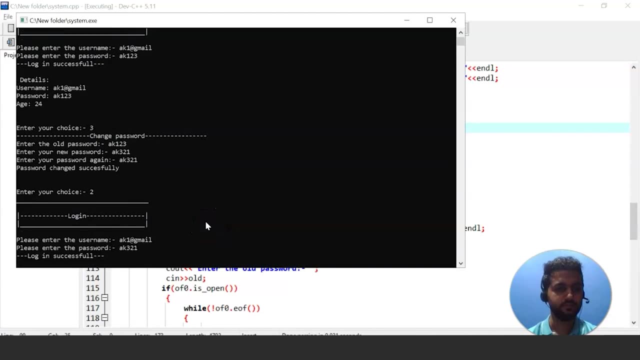 incorrect credentials. press two to login. press three to change the password. so now it's your choice. if you want to login again, then you can do that. if you want to change the password, you have to click on three and, as we know that, we know the right password, so we will not. 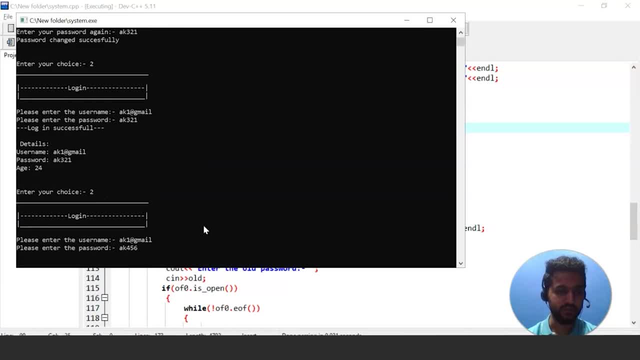 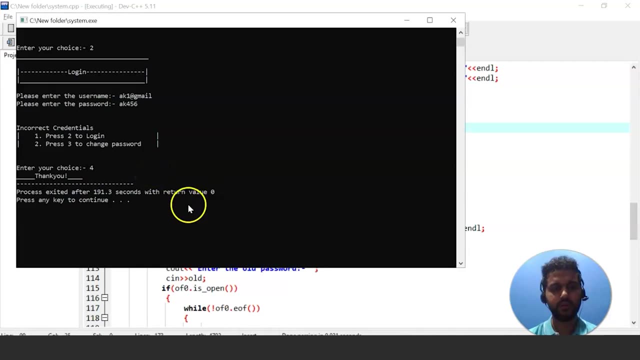 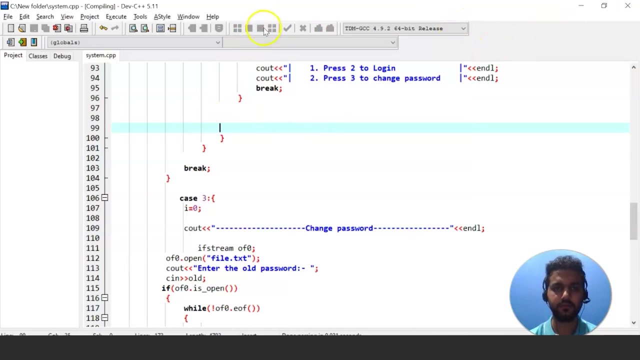 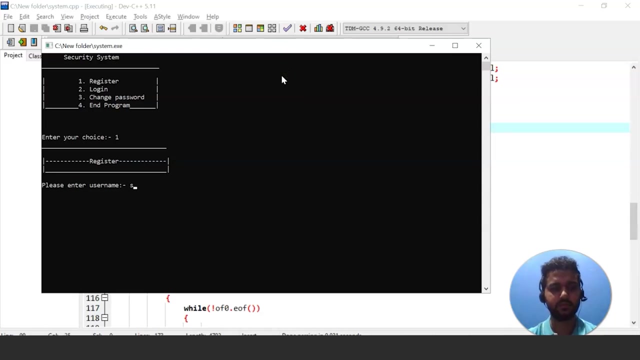 do that password change thing. alright, now we will click on four to end program. as we can see, thank you message is displayed. now we can also try one more thing, like let's try to run this again, as we can see. first of all, let's register. let's see: 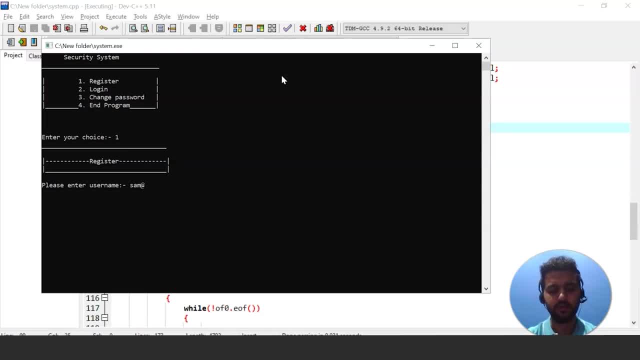 sam at the read: gmail. this is the username, the password is sam123 and the age is 24. so, as we can see, the registration is successful. now we will try to login. so while logging in, we will put the wrong password. let's see sam at the read. 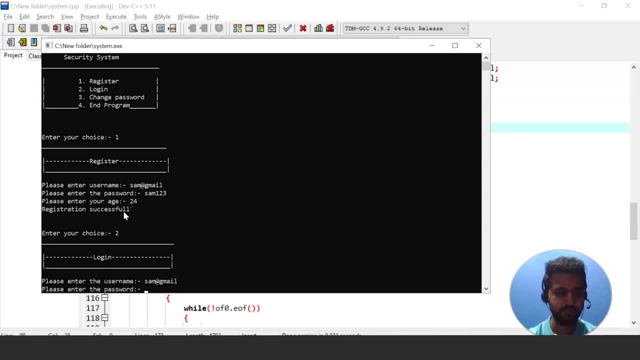 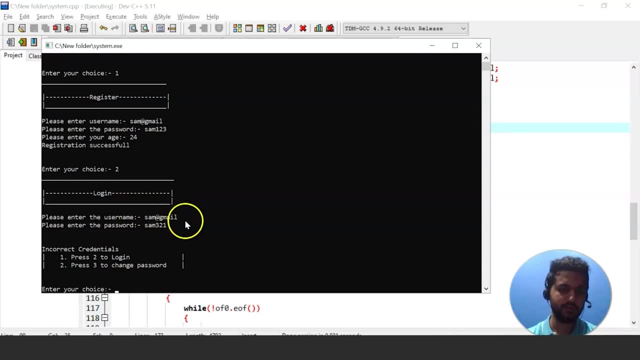 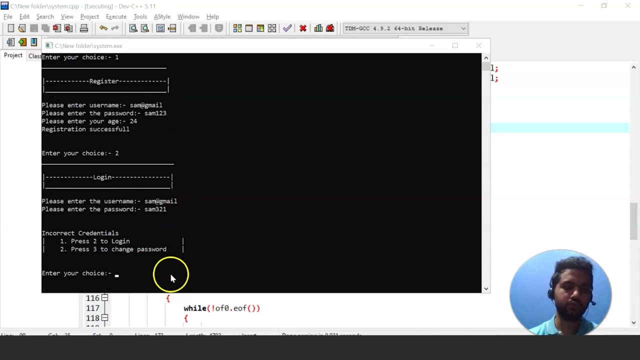 gmail, sam321. so, as we can see incorrect credentials again, press two to login and press three to change password, so you can click on two or three if you want to, if you want to login or change password respectively. i don't want to do that, so i will. 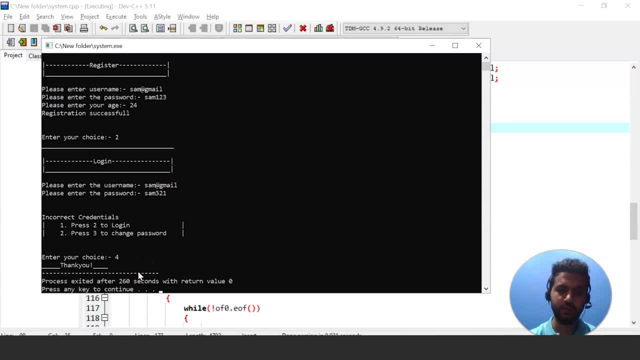 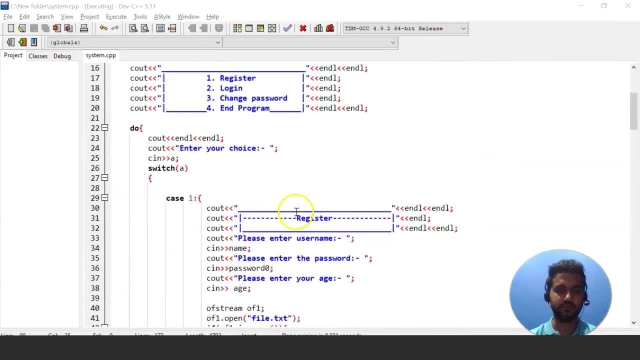 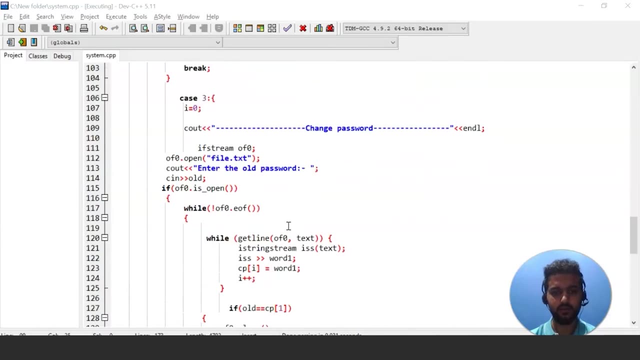 simply click on four to end the program. so thank you message will be displayed. so, guys, this was about this security system in c++. it is quite basic topic and all the concepts that are being used is intermediate level. you can create this on your own. you can add some. 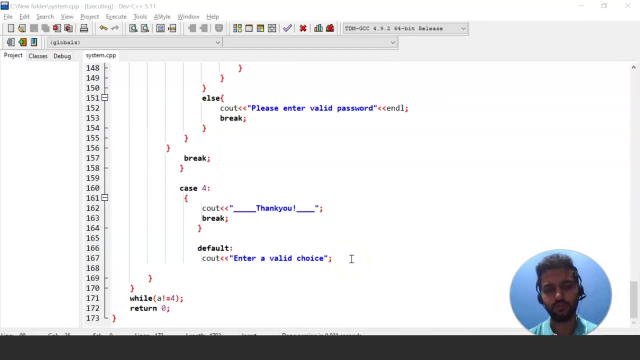 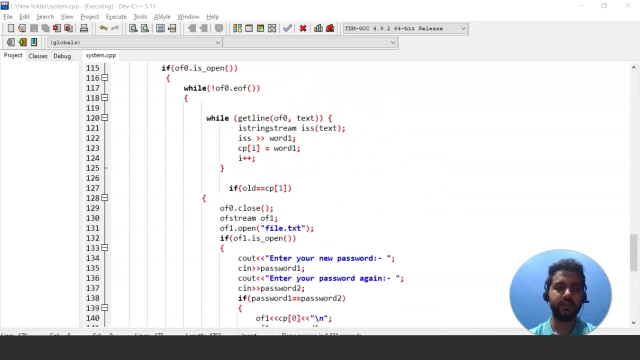 functionality, some more functionality to this security system also, and doing projects like this will enhance your knowledge in c++ and will give you, or show you, the practical aspect of c++. you can try this project on your own, and with that we have come to the end of this video on.